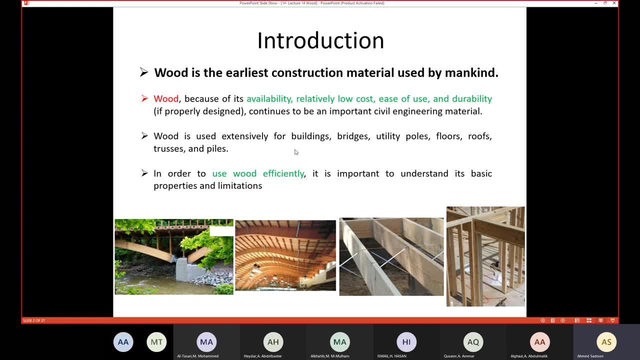 here. we have bridge, we have utility poles, we have floors, we have roofs, trusses and piles, so we could use wood in all of this. and in order to use wood efficiently, it's important to understand its basic processes. now i will show you how to use wood efficiently. 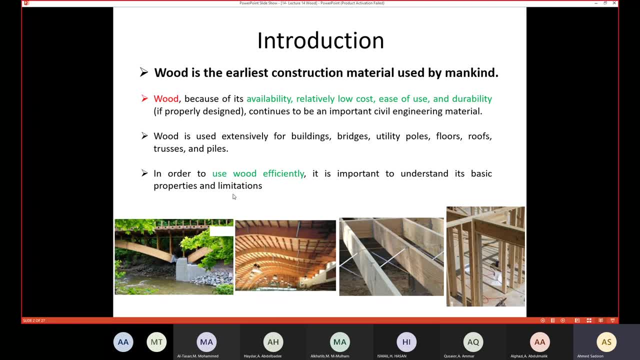 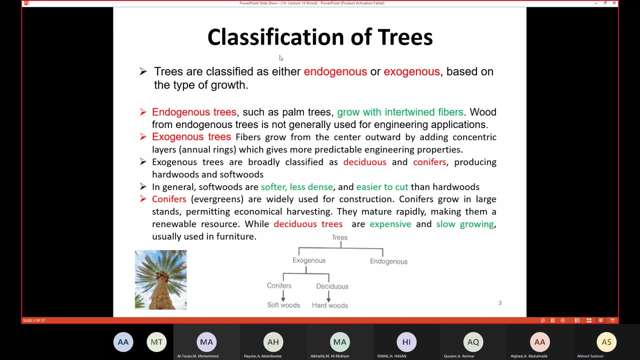 properties and limitations. So in order to understand how to use the wood, it's important to understand the properties and the limitations, like just any other civil engineering materials. So first we need to understand the classification of trees. We know that wood is made from trees. 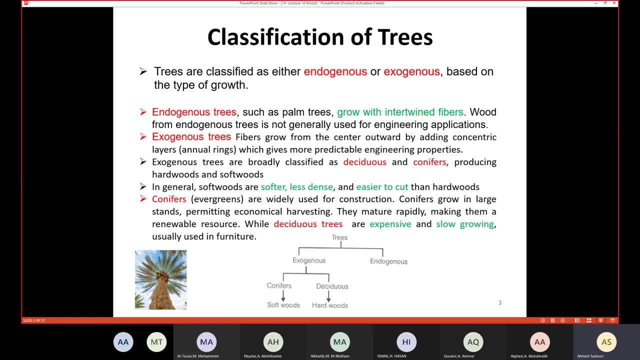 so we need to know the basic classification of the trees First. we have the endogenous, okay, and we have the exogenous. We have two main types. It depends on the type of the growth. First, what does it mean by endogenous? The endogenous trees such as palm trees like this. 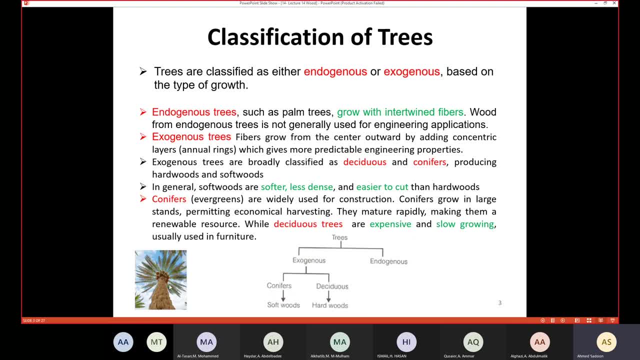 one. okay, we know the palm trees. In this type of the trees they grow with interwined fibers. So, like you can see here, they grow like interwined fibers And the wood, The wood from endogenous trees- is not generally used for engineering applications, So the trees- 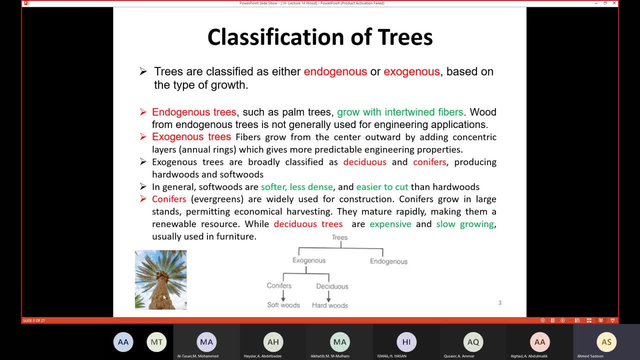 the woods from the palm trees. we're not going to use them in engineering applications. While the exogenous trees, the fibers grow from the center. So we're going, the fiber is going grow from the center outward, from the center then outside, by adding concentric layers. 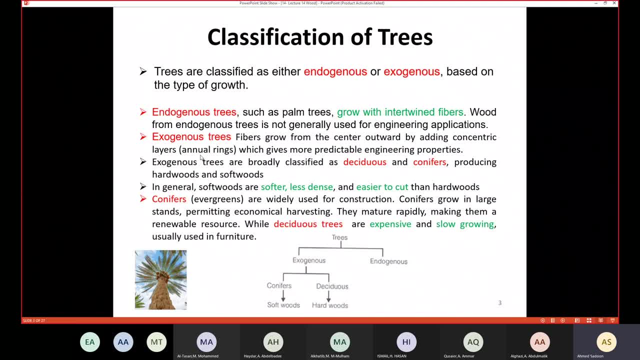 or we call this. we call these exogenous trees and we are going to use them from the hairline. So we use these exogenous trees from the center and then outside by adding concentric layers, And in order to use them, we need to make them more sensitive, okay. 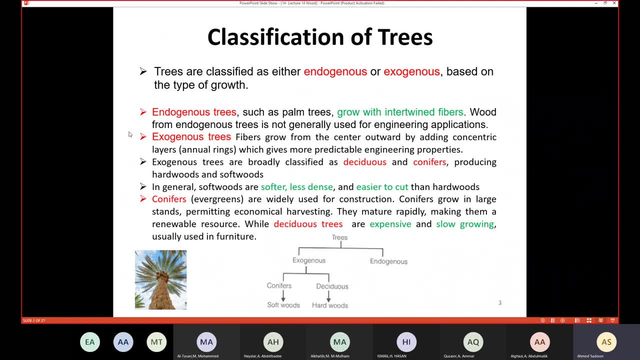 So the third type: we are going to use these in the linear unit and we are going to use them from the central. from the central, Okay, deciduous is going to produce hard wood, while the coniferous is going to produce soft woods. 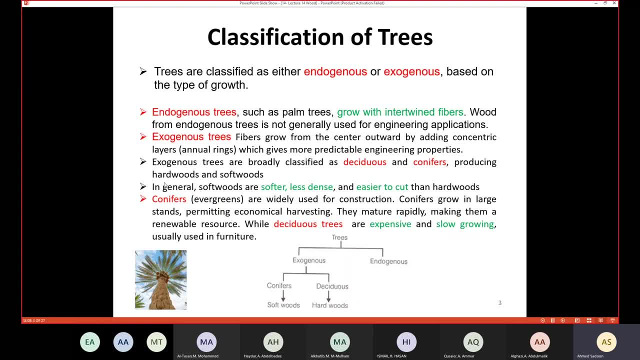 In general, when we say soft woods, it means that the trees is softer, less dense and easier to cut than the hard woods. Okay, so again here we have this chart show us the different types of trees. We have exogenous, we have endogenous. 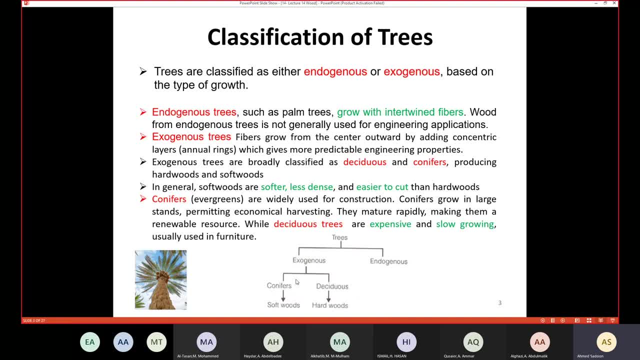 Endogenous, just like the palm trees Exogenous, this one which we use in engineering application. We have the coniferous, this one soft woods. We have the seduous, this one is hard woods, The coniferous also. it has other name, which is evergreen. 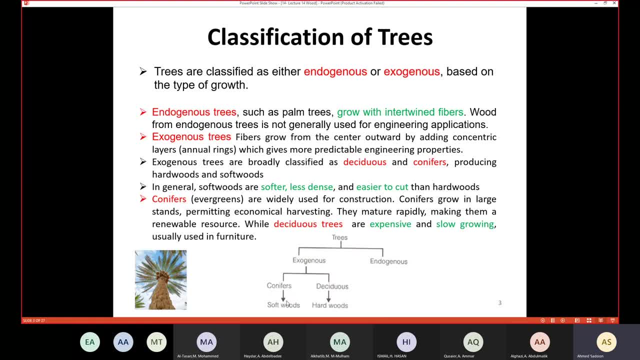 This one is widely used for construction. So the coniferous, this one is widely used in construction because this one, this one is widely used in construction, This one grow in the largest stands. The stand is going to be large and that is going to permit economical harvesting. 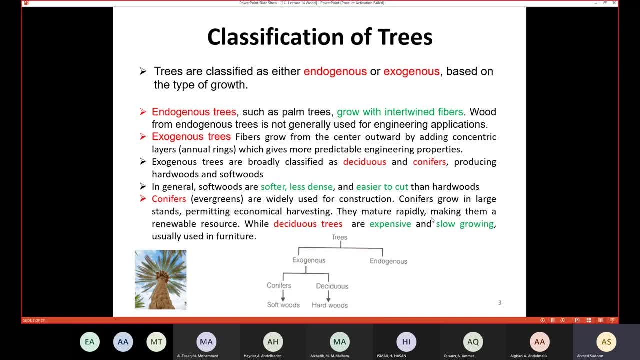 They mature rapidly and also which make them renewable resource. So in very short time they grow Okay, which means that if I'm going to cut the trees, I'm going to wait for a short time, then I'm going to get another tree. 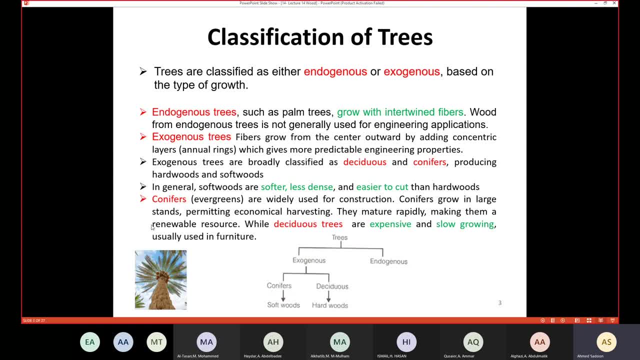 And that is going to make them renewable resource, While the deciduous trees- the other one here, this one is expensive and slow growing. It takes time in order to grow And we use this mainly in furniture. So the coniferous, we use them in engineering applications. 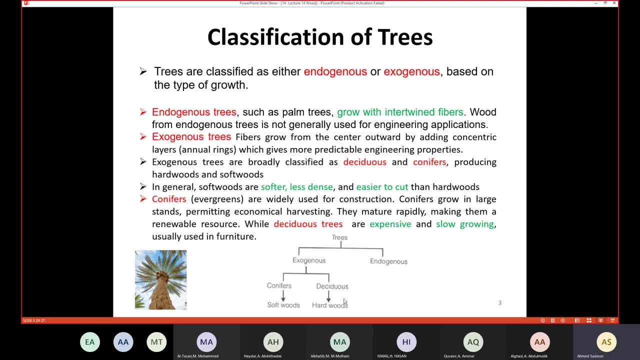 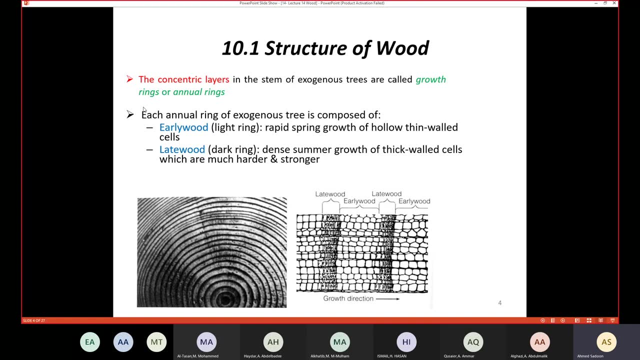 While the deciduous, we use them in furniture. This one is a hard wood, takes a lot of time to grow on it's offensive. This one is cheap and it takes less time to grow. Here it's important to understand the concentric layers. 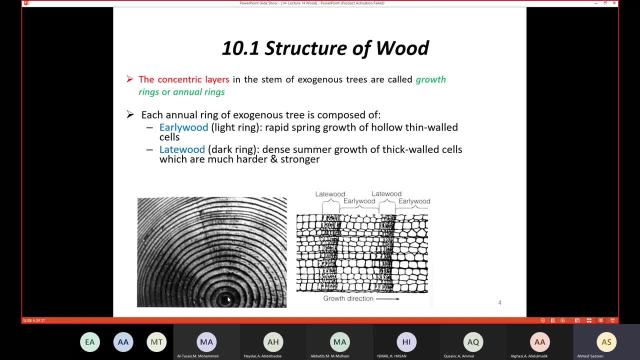 We say that the everything start, the fiber start from the center, and then we're going to have annual rings outward. Actually, if you know the numbers of the rings, you will be able to know the age of the tree. Okay, So if you have a specific age of the tree, that 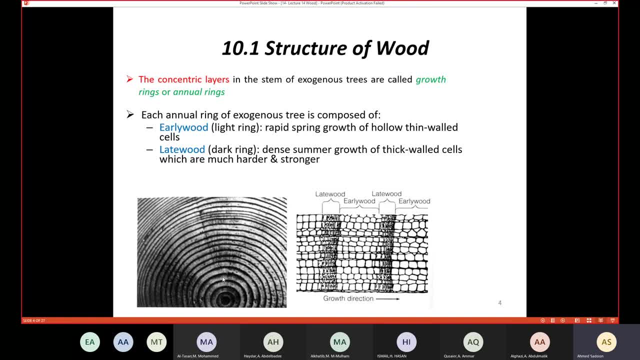 you will like. You can't use their appearance, but you can be honest, count the number of the annuals. you call this annual rings. so if you count the number of the annual rings, you will be able to know the age of the tree. so the concentric layers in the stem of 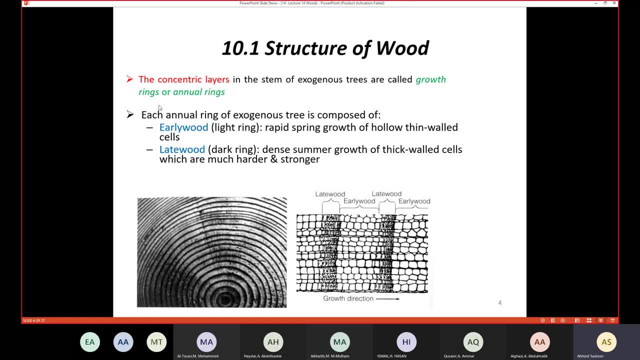 exogenous trees are called growth rings or annual rings, and the animal ring itself. it composed of two parts. we have the early wood or the light ring, we have the late wood. so each and every one of the ring it has two parts: have the early wood and we have that late wood. so if we are gonna cut small, 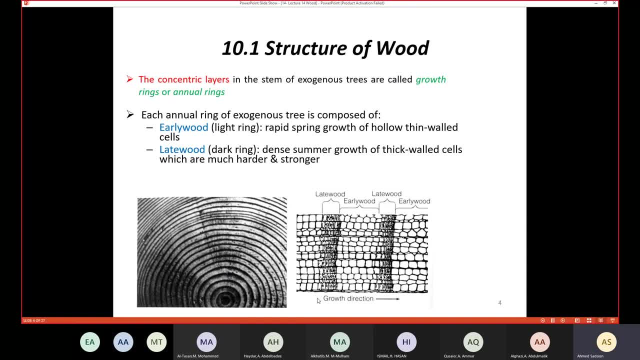 part here and assume this one is the direction of the growth. this direct, this is the direction of the growth, then we are going to have a late wood, then early wood, then late wood and early wood. the early wood, this one is a rabbit spring growth. it's going to rub it aggressively in the 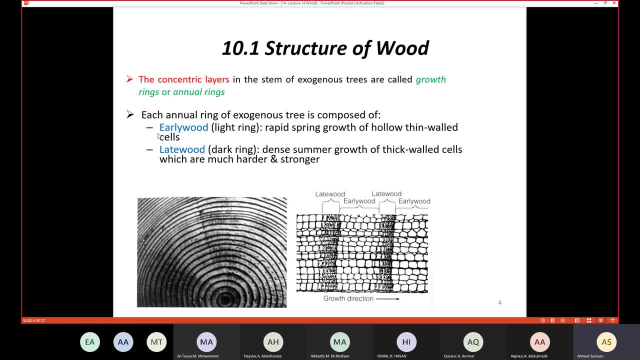 spring and it composed of hollow, thin wall cells. on the other hand, the late wood, dark green, this one is denser, summer growth of a thick wall cells which are much harder and stronger. so this one, much harder and stronger and darker. okay, and it's made from thick wall. 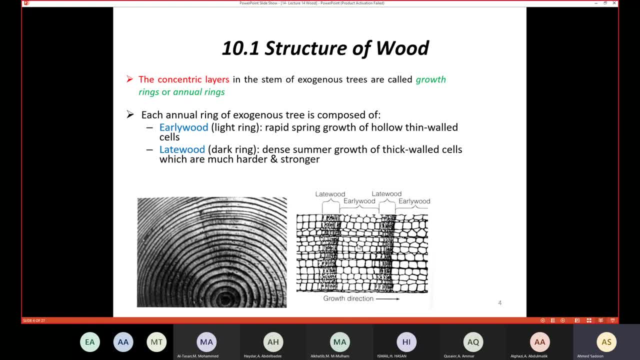 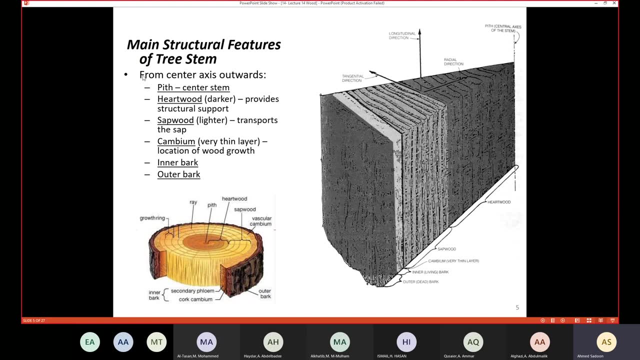 cells, while the early wood- this one is lighter and this one is a hollow, thin wall- this one grow in the spring and this one grow in the summer. also, it's very important to know about the main structural feature of tree stem. okay, we are going to start from the center. we say that this type of 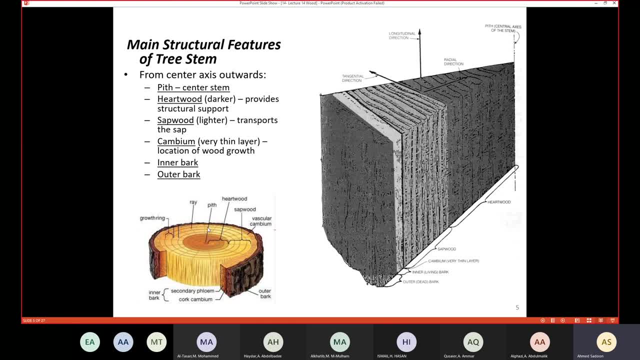 trees start from the center, then centric layers is going to be uh grown each year. so take a small slice here. this one- assume this one is the center- center is here. we are going to call the center the uh pith. so here we have the pith. 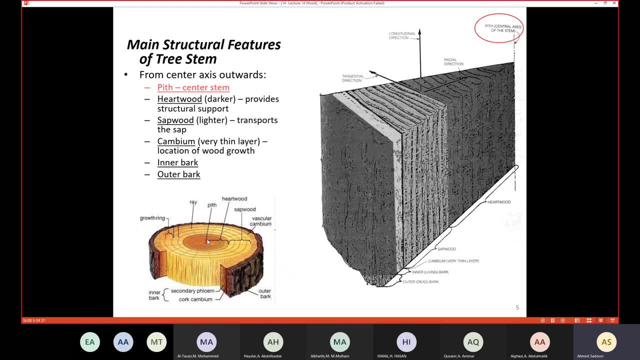 the center or the center stem of the the tree. then we are going to have the heart wood. this part here is the heart wood and this one is the darker. and this one provide structural support for the tree, so the tree take its structural support from the hard wood. then we are going to have the sap wood. this one is the lighter. 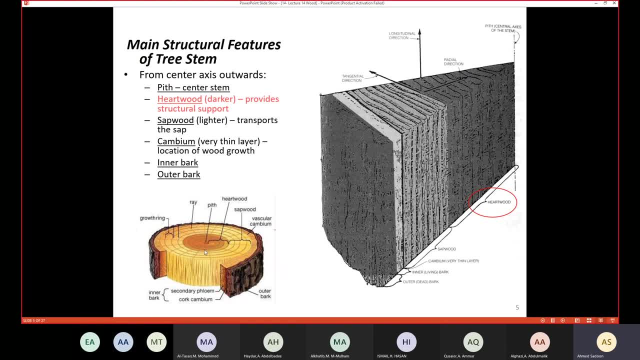 okay, and this one is going to transport the sap, the food of the of the tree. okay, then we are going to have the cambium. the cambium is very thin layer. so here we have the hardwood, this part, then we have the, the sap, and then we have the cambium. cambium is a very thin layer. 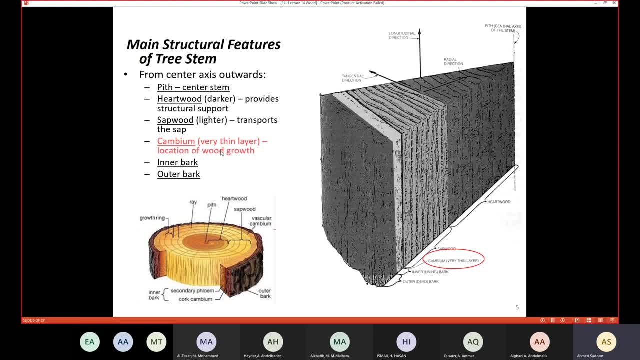 okay, this is the location of the wood growth here, where a new annual ring is going to be created. finally, we have the bark bark. we have the inner bark and we have the outer bark. the bark itself- we have the inner bark and we have the outer bark- is the main structural feature of the tree stem. 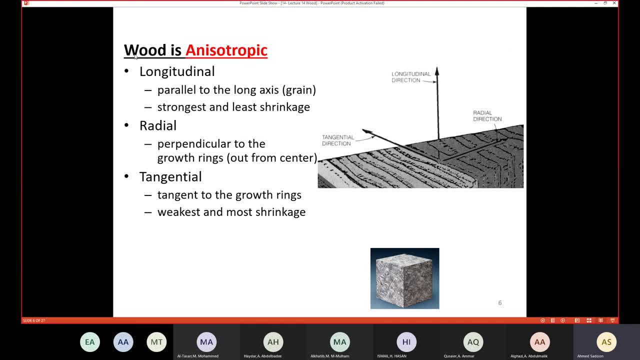 and it is very important to know about one of the most important information, information about the property of the wood. the wood is anisotropic. okay, this strange, and i think this is the first time for you to find something or material like this. remember when we dealt with the strings of material before we bark on any definition or differentiation. 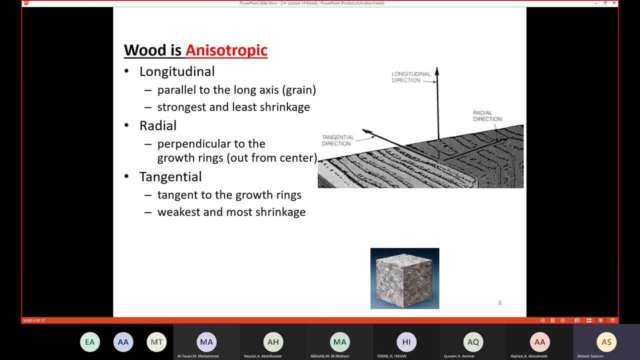 or any something like that. we are going to say that the material is going to be plastic and the material is isotropic, and so on. before the starting, the derivation is going to give you some information. one of the of the information: they will say that the material is isotropic. 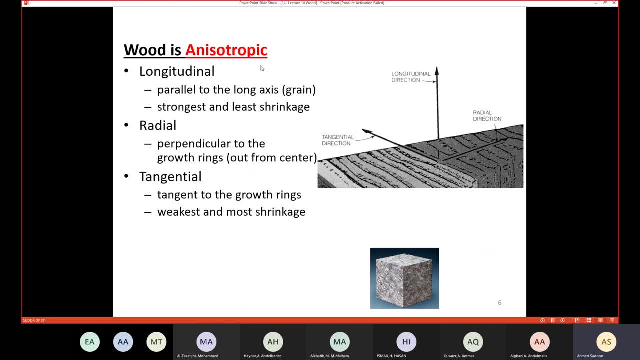 so what does it mean by isotropic and anisotropic? so, for example, if you have a cube here made from concrete, for example, if you are going to apply, if you want to test the compression, compressive strength, for example, now you apply, you apply the load from this direction, for example: 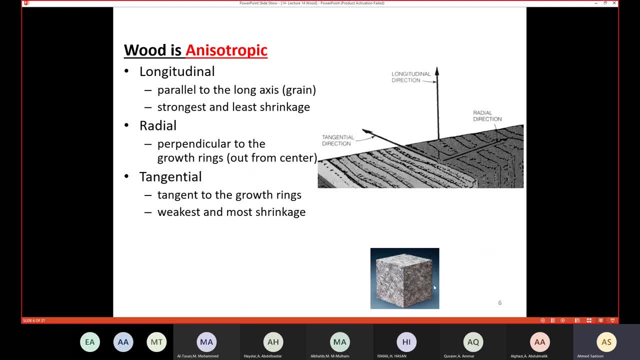 okay and you fix this part and you apply a force from here. you got the value. what if i apply the load from that direction and fix the value or someone else is going to fix this part here and apply the load here? will it make any difference? of course it's not going to make any. 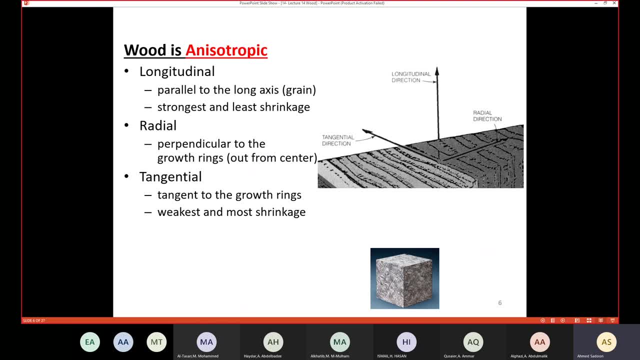 difference. right, even if you have a small difference is going to be very small. so this is not the case for the wood. the wood: any direction, it has different properties. any direction it has different properties, not like the steel or concrete or something like that. this is different from any. 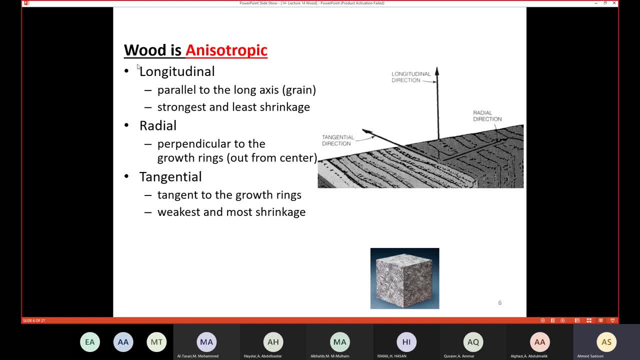 other material. that? what does it mean by wood is an is an isotropic. so in the wood we have three main directions. we have the longitudinal direction. this one is parallel to the long axis of the tree. so if you have the long axis of the tree, the longitudinal is going to be parallel to. 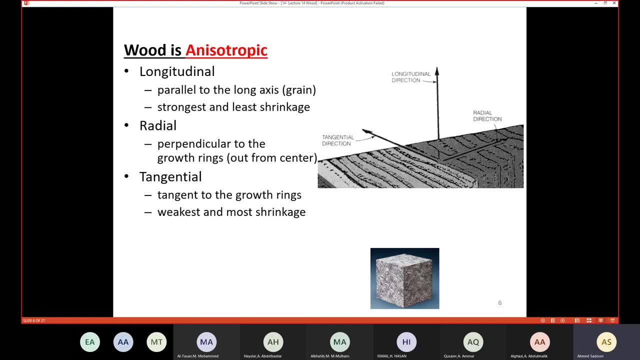 the long axis. this one is the strongest axis and the least shrinkage, so this one is not going to have reduction in the volume or is going to went through a small reduction in the volume. then we have the radial direction direction. this one is perpendicular to the growth rings. so if this one is the growth link rings, 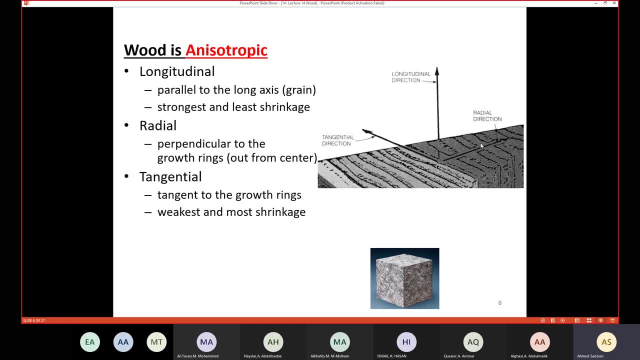 then the radial is going to be perpendicular to the growth rings. okay, uh. finally, we have the tangential. this one is tangent to the growth length, so this one is going to be tangent to the growth links. this one is the weakest and the most shrinkage. okay, so, uh, when we say wood, 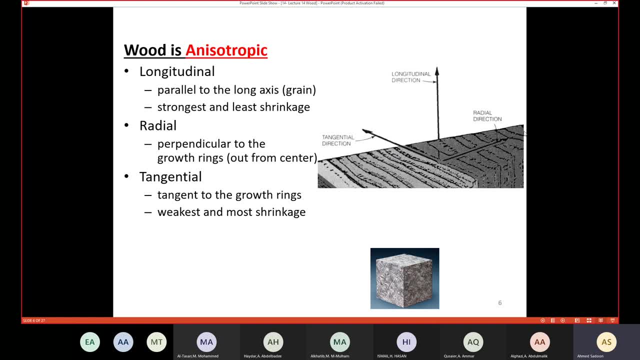 is anisotropic, which means that the properties in this direction is different than the properties from that direction and it's different from the properties of that direction. okay, that is why the wood is unique material, so the properties is going to change with the direction. that, what does it mean by anisotropic? yeah, here i have the longitudinal. 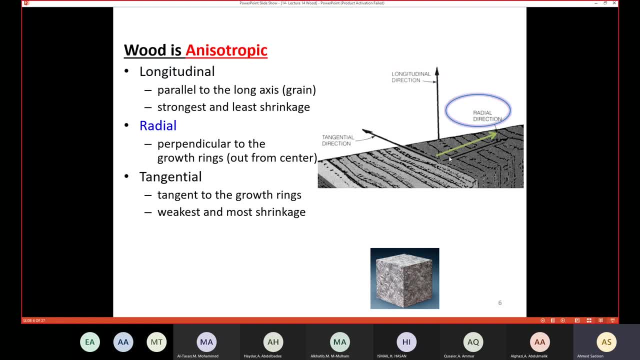 direction. here i have the radial direction. this one is perpendicular to the growth link ring. here i have the tangential. this one is tangent to the growth rings. so in the wood directions influence strength, modulus of elasticity, thermal expansion, conductivity, shrinking and extra, etc. it is going to affect many properties. 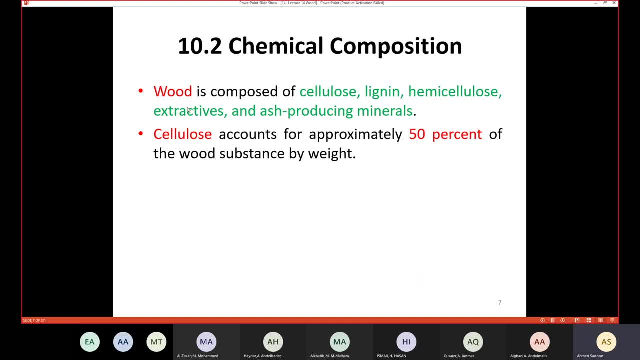 then we have the chemical composition of the wood. wood is composed of cellulose, okay, and we have lignin and we have hemice cellulose, we have extra extraffitis and we have ash producing minerals. so here the wood is composed of many chemical compounds, but the 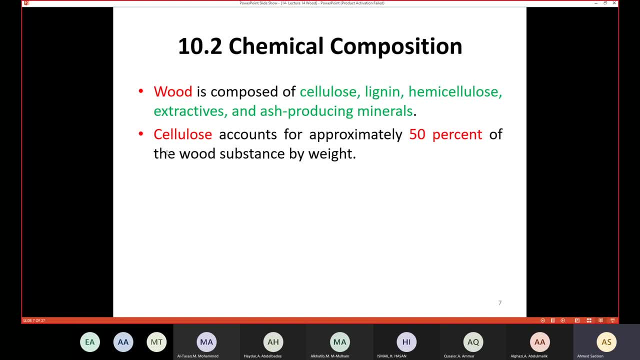 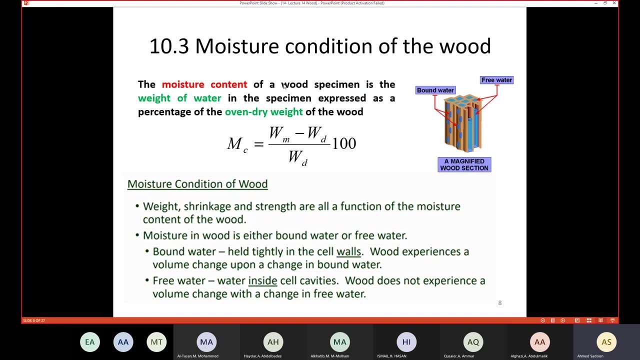 powerful theory of lignin and heme. cellulose is the account for approximately 50 of the wood substance by weight, so this one is the most important chemical part of the wood. also, it's very important to understand the relation with the moisture condition of the wood. 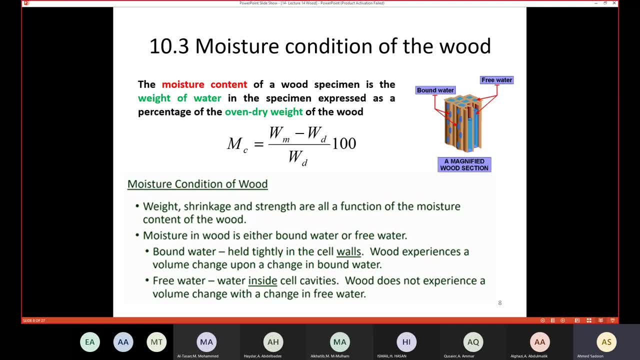 in the, when we discussed the aggregates, for example, we discussed the moisture condition. uh, we say that the aggregate, it, has voids through which it can absorb water. okay, so here also, the wood can absorb water. so it's very important to understand the moisture content for a specimen of a wood. so how i'm going to determine, 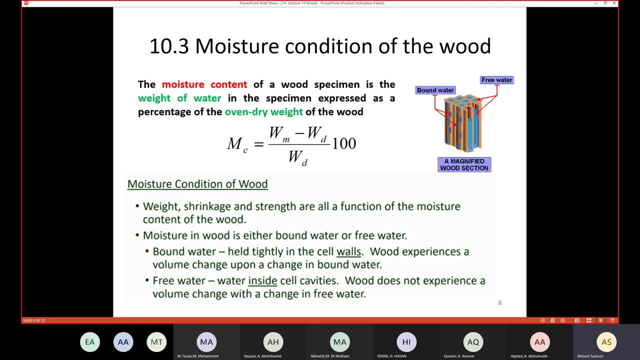 the moisture content for a wood. so if you have a small piece of wood, then the moisture content is going to be the weight of the wood minus the weight of the wood dry over the weight of the wood dry. so you are going to take a sample from the wood with its water. okay, you are going to. 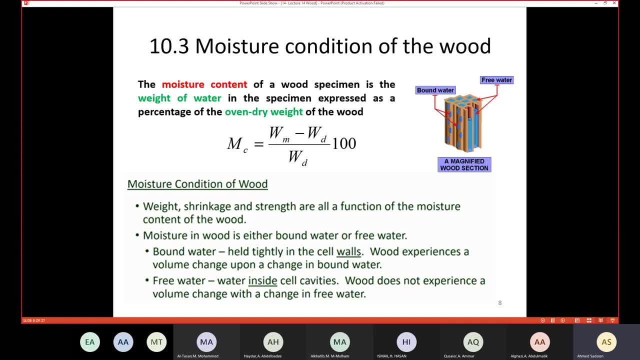 measure it, then you need to put the sample in the oven so that the sample is going to be completely dry. then if you substitute w m minus w d d, you are going to get the water content. then divide it by the weight dry, then you are going to get the moisture content. you need, of course, to multiply. 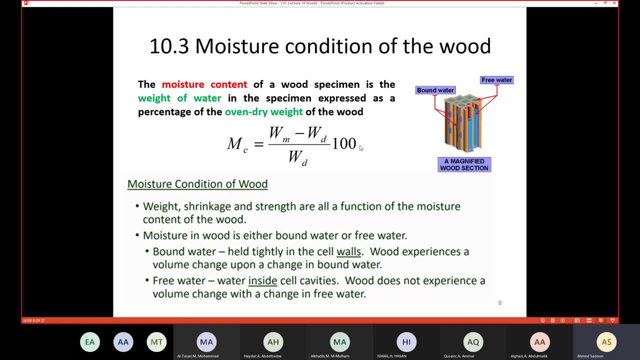 by 100 percent to convert it to be a percentage. the moisture condition of the wood, the weight, the shrinkage and the strings are all function of the moisture content of the wood. also, the moisture content is going to affect many properties of the wood. but we need to understand the types of the moisture. we have two types of moisture in. 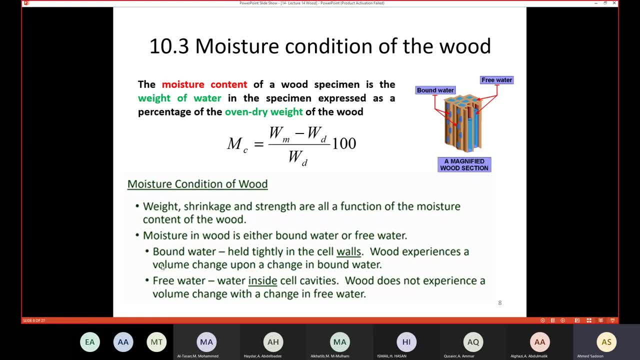 wood. we have bound water and we have free water. here we have a magnified wood section, like you can see here. we have water on the war cellsand. we have water and we have free water. we have wateron the wall sels. washing is very important, as you can see here we have free water and when this happens, water carries beautifulavors like this. everybody can receive a sac and an growngery like this which were used for sleep 여기. this is a covered water. WE can see here we have leisure. we can reach the top here, on top of the wall cellsand, we have water on the space. here is water on the wall cells and we have water above the walls and we have water above the walls Also, for example, On the dried conditions. we can be under water on the floor. 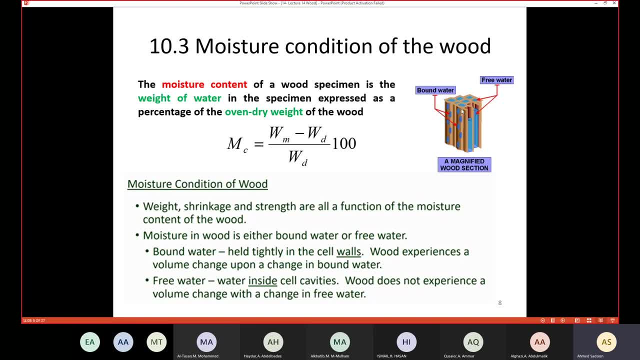 and we have water inside the cell cavities. we have two types of moisture content: one inside the cell cavities and one in the cell walls. okay, we call this bound water and we call this free water. so the bound water held tightly in the cell walls here and the wood experience. 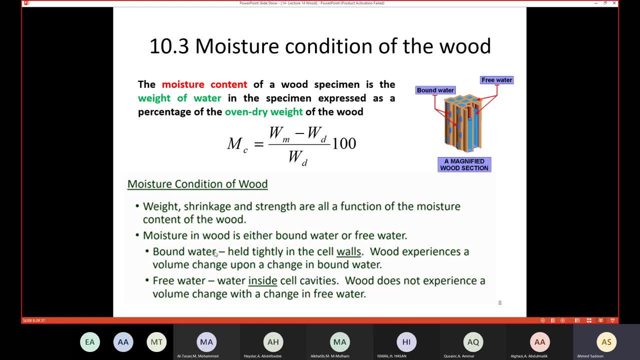 a volume change upon a change in the bound water. so any change in the bound water, then we are going to have a volume change accordingly, okay, while for the free water, the wood does not experience a volume change with a change in free water. so if this free water is going to change, the wood is not going to 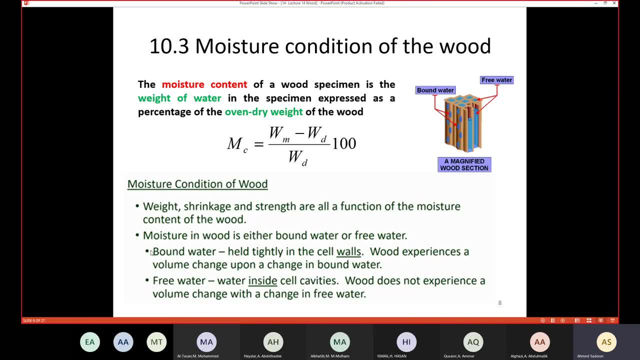 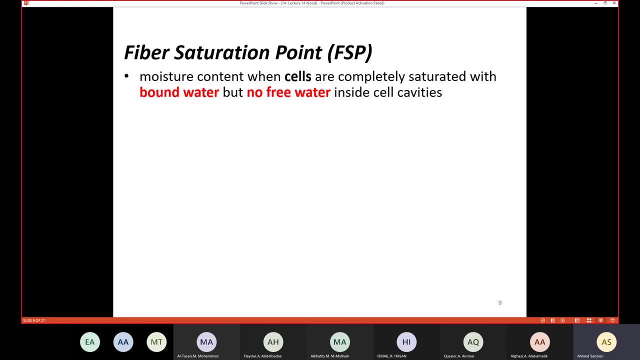 experience any volume change is the difference between the bound water and the free water and their effect on the volume change. in the wood also we have the fiber saturation point fsb. okay, the moisture content when cells are completely saturated with the bound water but no free water inside the cell cavities. so in this case we have bound water. 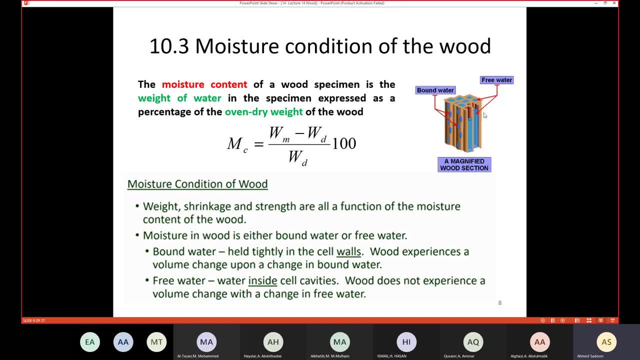 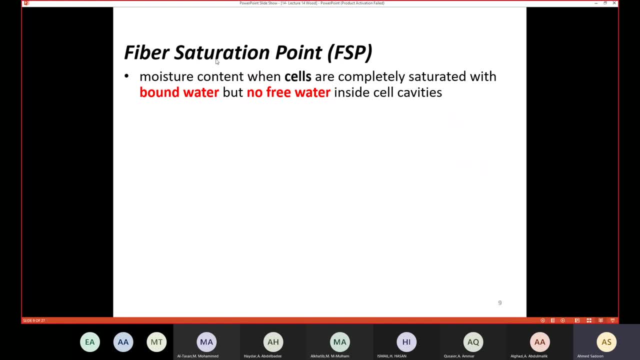 the wood is saturated with the bound water but we don't have any free water. we call this moisture content, fiber saturation point. okay, so again, the bound water, uh, the held tightly in the cell cavities, would shrink, shrink, shrinks on removal. so if you, uh, if we lose or we remove any amount of bound water, 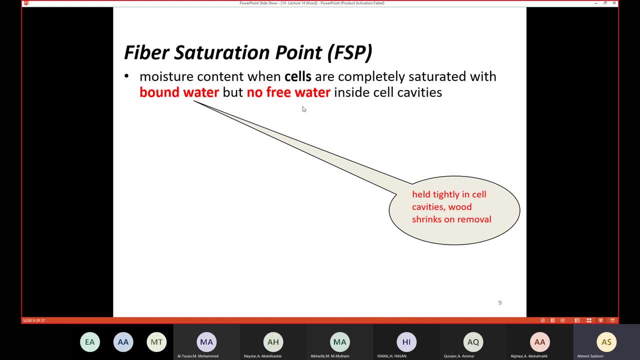 then we are going to have shrinkage, not like the free water, while the free water- water inside the cell cavities- does not affect the shrinkage. you already mentioned this. the uh fsb, the fiber saturation point, is going to be between 21 and 32 percent. so see uh moisture content. so it's 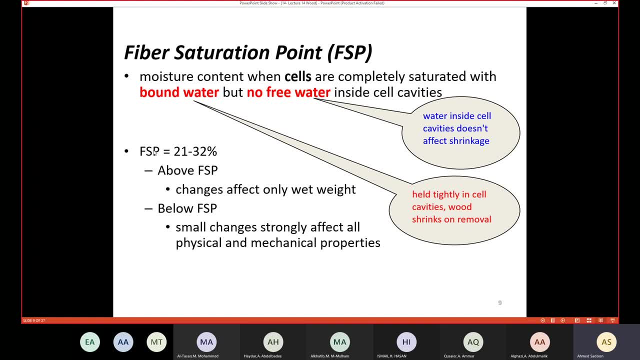 going to be between 21 and 32 percent. so if the moisture content above the fsb, that is going to change uh only the wet uh weight of the uh wood. okay. and if it's below the fsb, then small changes affect all the physical and mechanical properties, okay. so if the moisture content above the fsb, 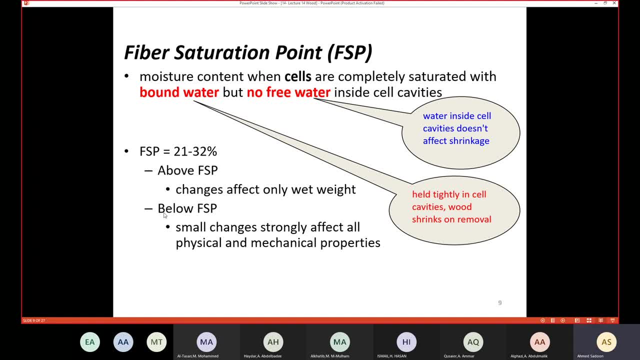 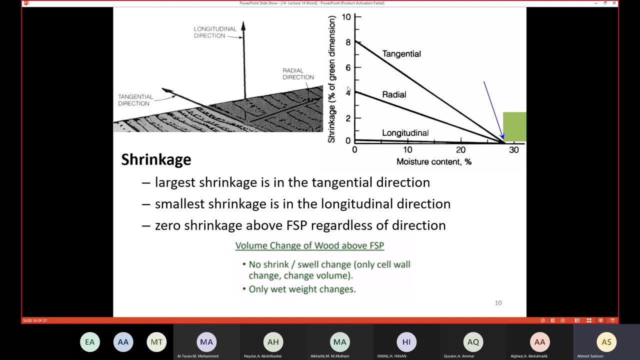 changes affect only wet weight, while if it's below the fsb, then small changes- even if you have small changes- strongly affect all physical mechanical properties. so here we have this graph in order to understand the relation between the moisture content with the three main axis. we say that we have the longitudinal direction. 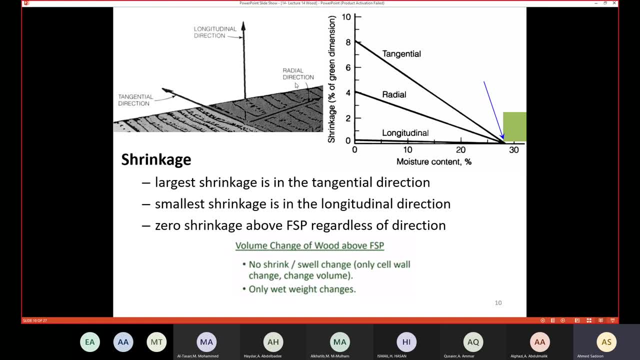 we have the tangential direction and we have radial direction. here we have tangential radial and longitudin. alright, here we have the moisture content in the x axis and in the y-axis we have the shrinkage. okay, like you can see here, when the uh, the value of the 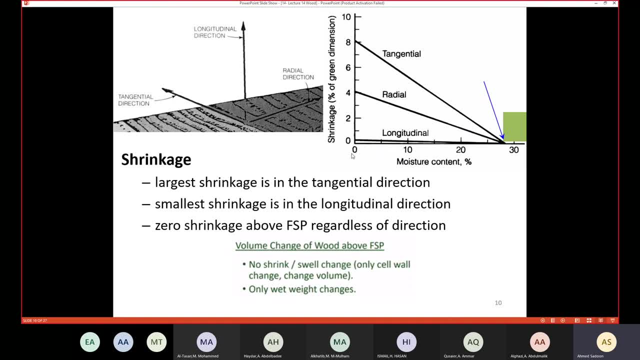 content is zero, then the percentage of the shrinkage is high, actually is very high in the tangential direction and it's medium in the radial direction and here it's almost zero in the longitudinal direction. then when the moisture content increase, the value of the shrinkage is. 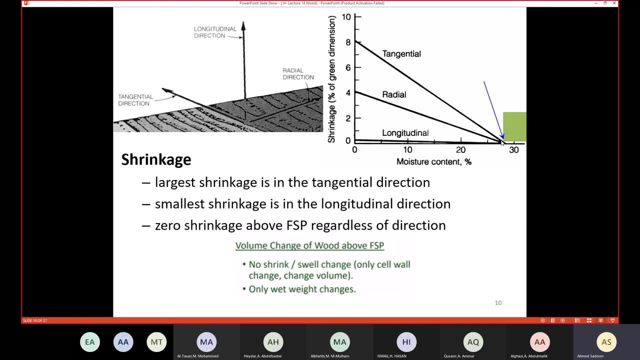 going to decrease and when we almost got at at the fsb point, the fiber saturation point, here, then the shrinkage is going to decrease for the all direction. but like you can see here, the tangential direction, like we mentioned earlier, is going to be affected strongly. 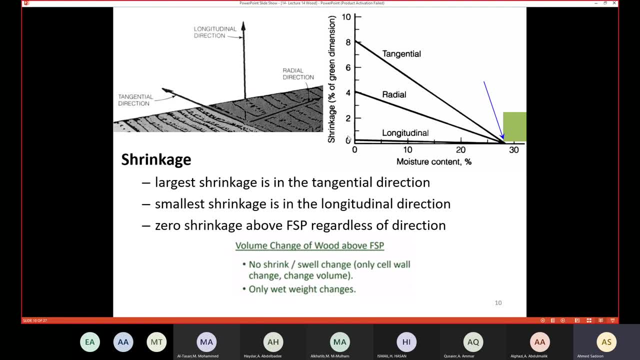 by the moisture content, not like the longitudinal direction. that is why we say that the wood is anisotropic. they are going to be affected differently in different directions. so largest shrinkage is in the tangential direction. so this one is going to experience the largest shrinkage when we have a change in the moisture content. 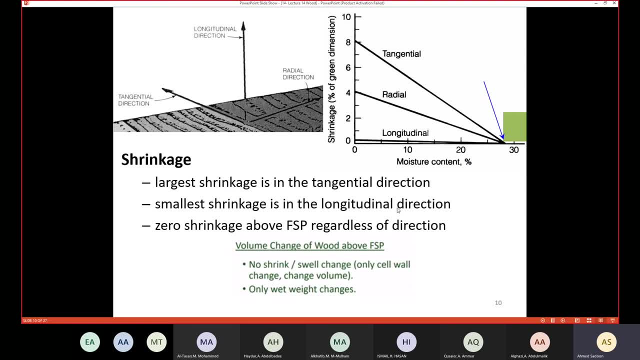 and the smallest shrinkage is in the longitudinal direction. this one is going to experience the smallest shrinkage, okay, and here we are going to have zero shrinkage above the fsb. so after the fsb point we are not going to have any shrinkage, whatever the direction. 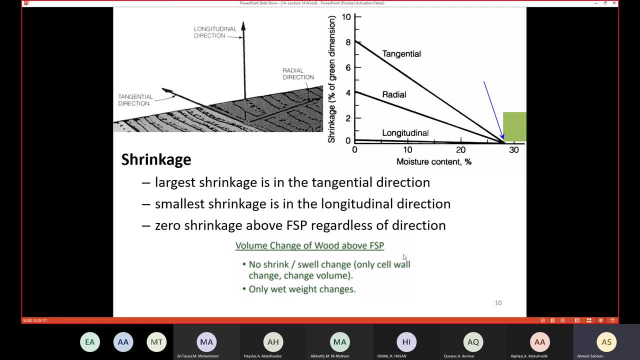 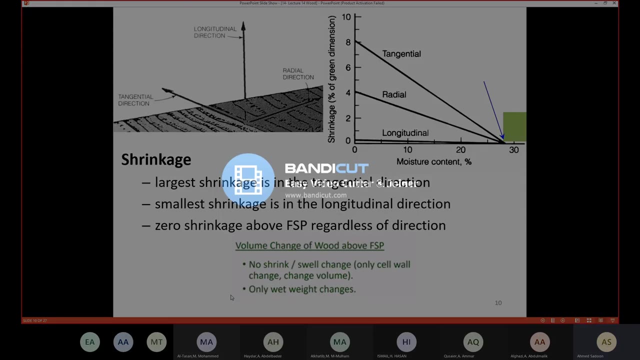 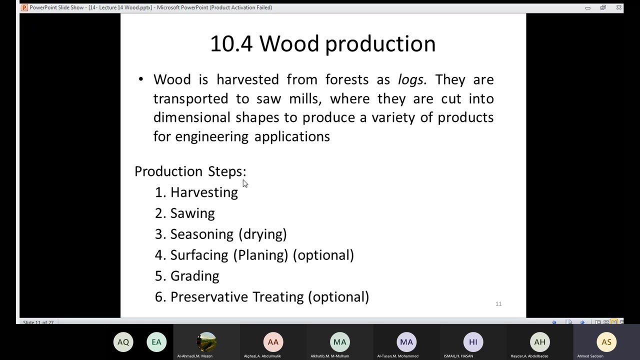 okay. so volume change of wood above fsb, no shrinkage as well. change only cell wall change. change in volume we have only with weight changes. okay, so after the fsb we have only with weight changes. in the wood production we have many steps. first we have the harvesting, then we have the 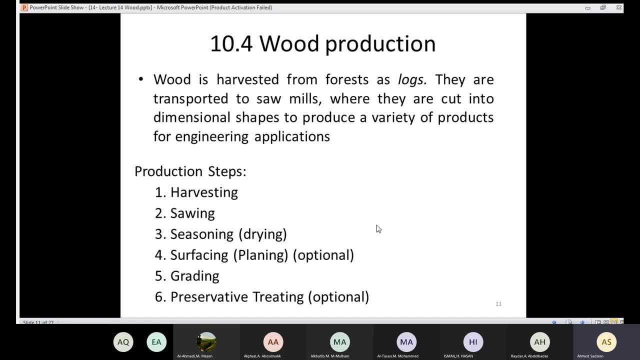 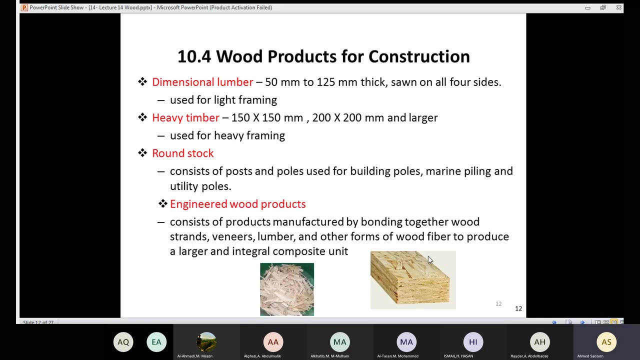 sewing, then we have the seasoning or the drying, then we have the servicing or the planning. this one is optional. we have the grading and finally, we have the pre-servitive treating, this one in order to prevent the insects and the fungi from degrading the the wood. we have wood products for construction, like the dimensional lumber. look. 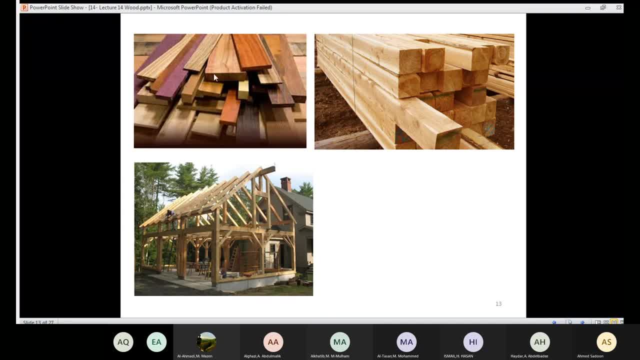 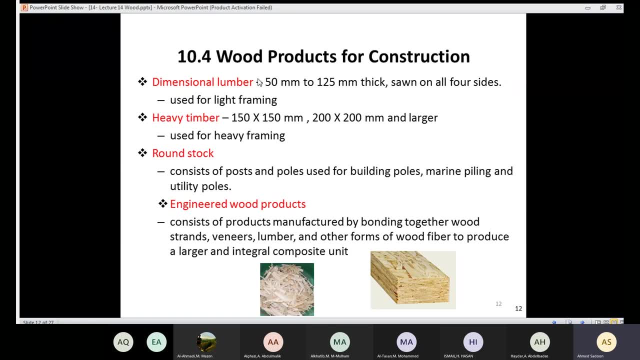 like that. this one is the dimensional lumber. the size is small compared to other it's. it has a thickness between 50 millimeter minimum to 125 millimeter maximum, and this one is going to be sewn on all four sides, so the fall four sides is going to be sewn. 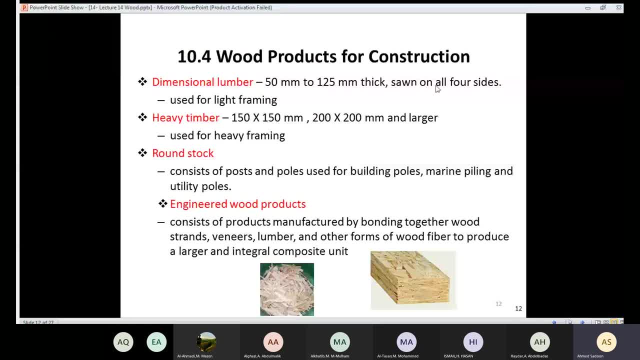 okay, and this one used for light framing. so if you are going to have light framing, then the lumber is a good option for you, but if you want to construct heavy framing, then you need to use heavy timber. in this one, the cross section is going to be 150 by 150 or 200 times 200. 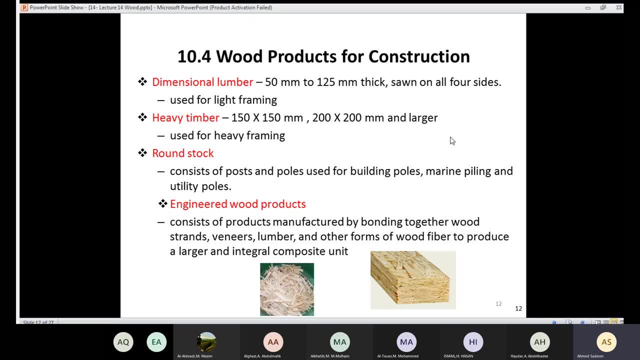 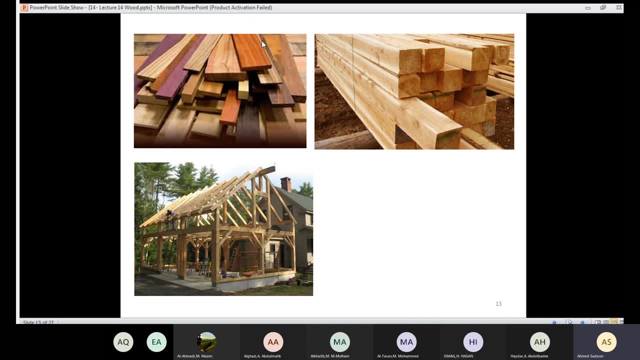 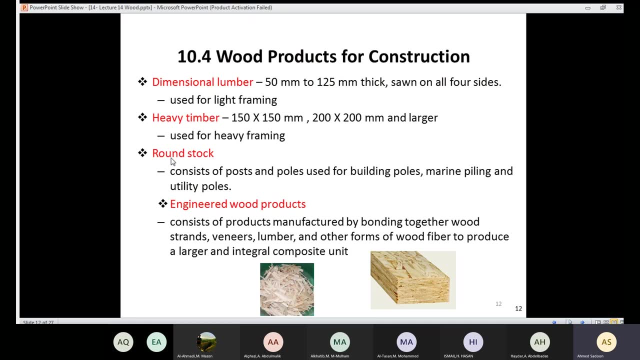 millimeter or larger, like this one here. this one is is larger than that one. we use this one for heavy framing, while this one for light framing framing. also, we have the round stock. this one consists of post and poles and this one used for building poles, marine piling and utility holes. so we use this one in places like here, maybe in. 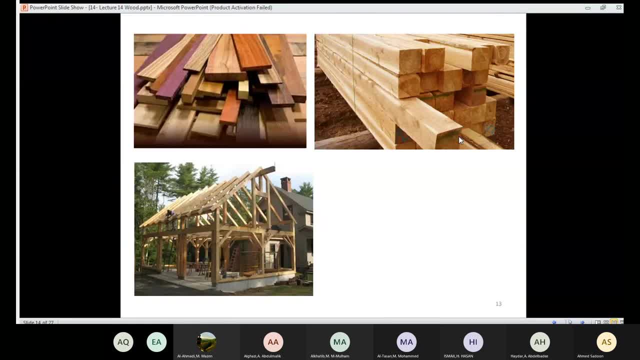 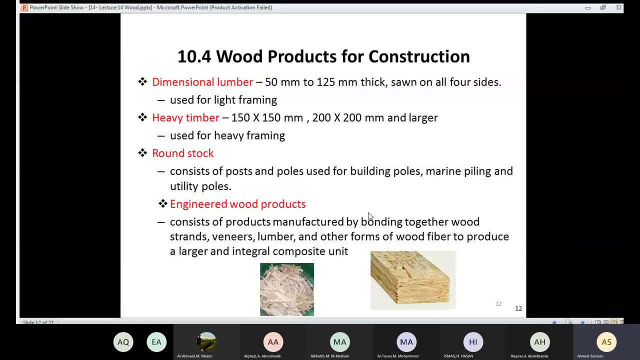 the center or something like that. finally, we have the engineer wood products. this one consists of products manufactured by bonding together wood strands and the other one consists of the wood fibers. so we are going to make bundles of the wood for wall and as a form of wood fibers, so we 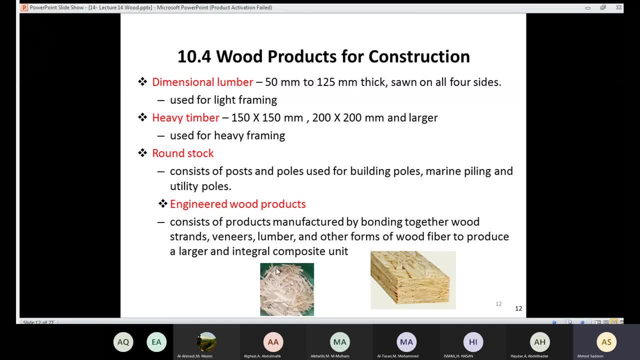 you are familiar with wood fiber like this one, then we are going to bond them together, put them, put them like that and we call this engineering wood products. like the playwood is a famous one, famous engineered wood products. so we are gonna get benefits from the strands and the veneers. 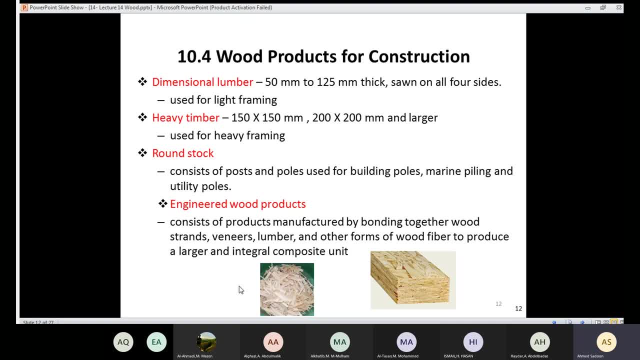 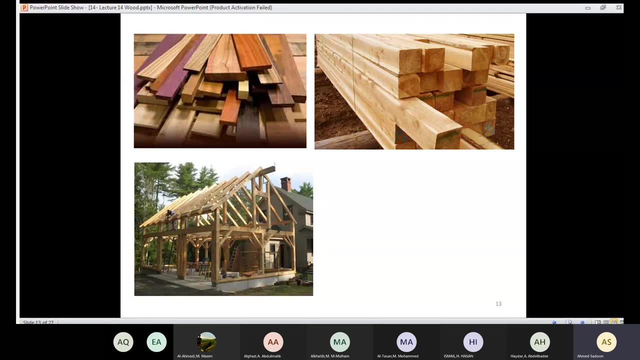 we are going to bond them, to get together by chemical boundary so that they are going to take this shape. nowadays the the use of engineered wood products becoming a lot. here we have a pictures. here we have a pictures for lumber and heavy timber and here we have a picture for frame. this one is a heavy frame, not light frame. here we have many. 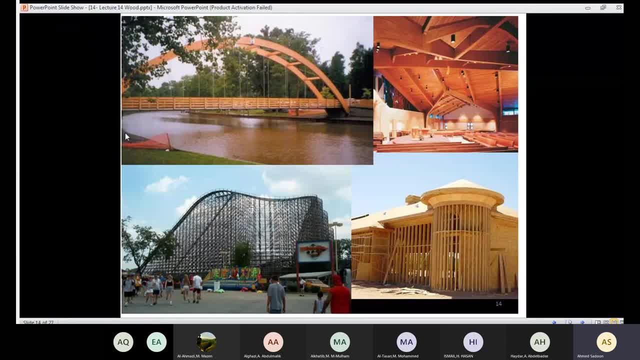 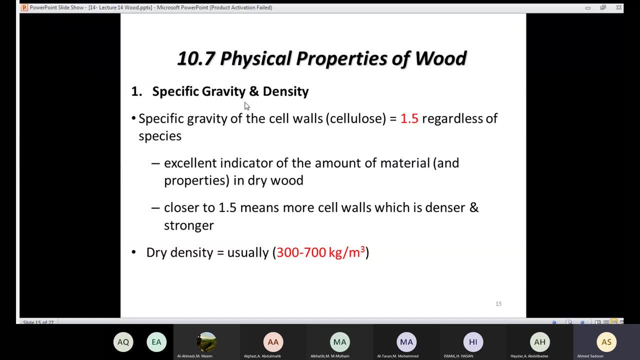 applications have been done using the, the wood. now let's talk about the physical properties of the wood. first, we are going to talk about the specific gravity and the density. the specific gravity of the cell would, in Celsius, is 1.5, regardless of the species, so regardless of the 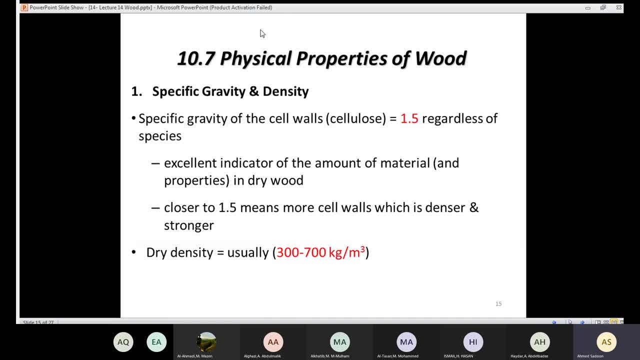 species, whatever the type of the tree, the cell would is going to these Celsius. specific gravity of the Celsius is 1.5.. point five and the specific gravity, excellent indicator of the amount of the material and the properties, especially in dry wood. if the value is close to 1.5, the specific gravity of the dry wood. 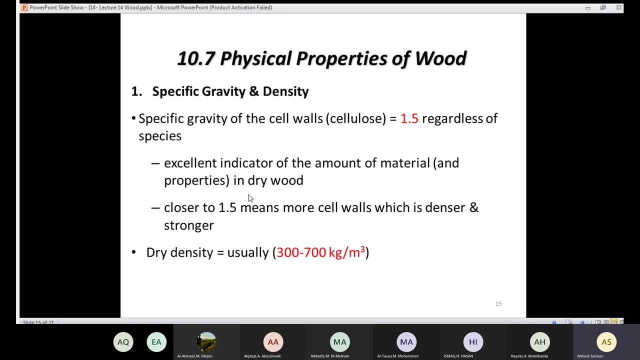 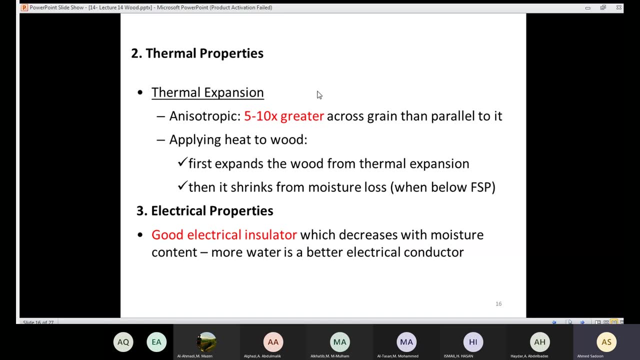 is close to 1.5 mean it means more cell walls, which is denser and stronger. and regarding the density, the density between 300 to 700 kilogram per cubic meter, and also we have the thermal expansion. uh, previously mentioned that the wood is an isotropic material, which means that the 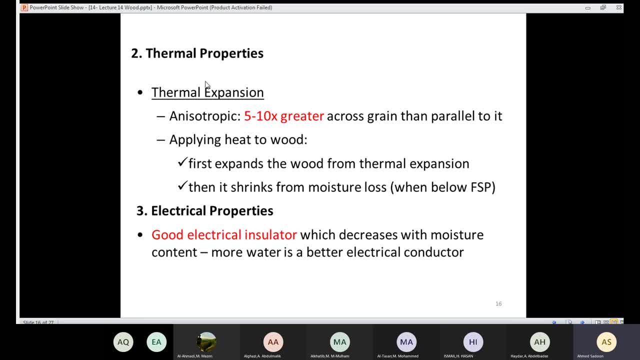 properties differ in each direction. and regarding the thermal expansion, about five to ten times the thermal expansion is greater across the the grain than pearl to it. so across the grain the thermal expansion is between five to ten times larger across the grains on the other direction. so when you apply heat to wood, what will happen we have first, the wood is going to expand. 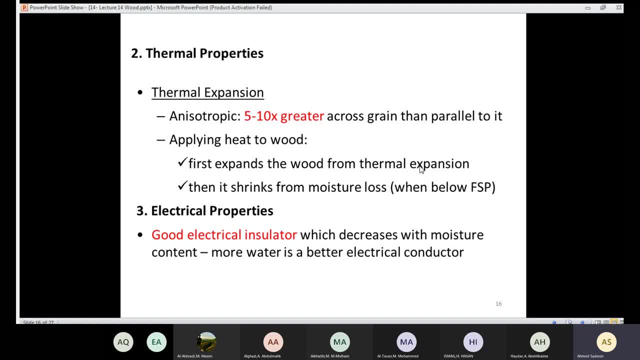 from the thermal expansion. the length is going to increase, then is going to shrink from the moisture loss. then, after a while, the wood is going to suffer moisture loss and the value of the moisture content is going to be below fsp and in this case the uh. the wood is going to 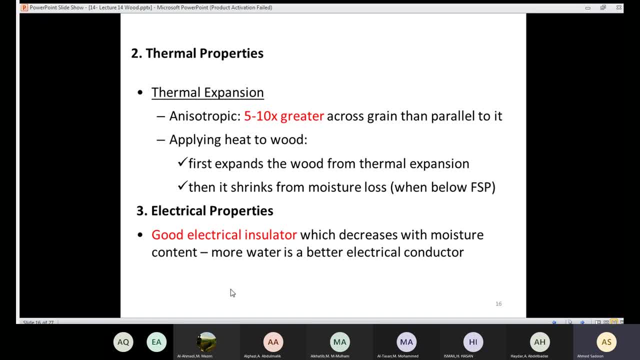 shrink again. and regarding the electrical properties, the wood is a good electrical insulator in general, but that is going to be affected by the moisture content. more water is better as electrical conductor, so if the the moisture content increase, then the wood is going to be good electrical conductor. if the moisture content is decreased, then the wood is. 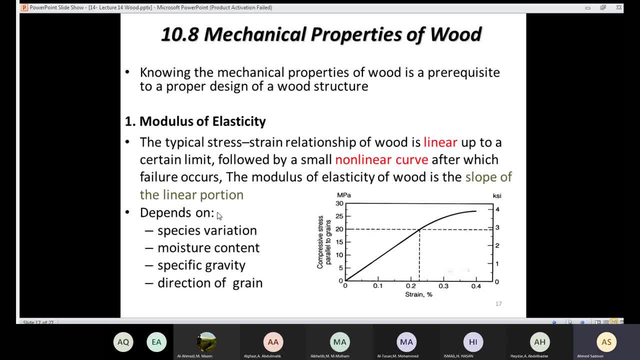 going to be good electrical insulator. regarding the mechanical properties, the mechanical properties is very important. we have done, and or we have seen how to conduct mechanical properties for different type of material. this time we need to know the mechanical properties for the wood. so in order to 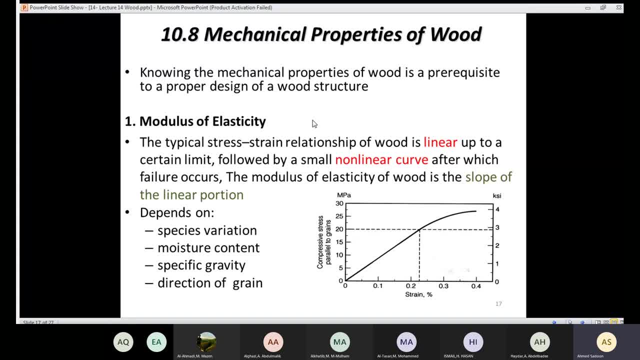 design the wood, you need to understand the mechanic, mechanical properties. so we could say that the mechanical properties is just like a prerequisite for a proper design of food structure. first we have the modulus of elasticity. we know that in order to get the modulus of elasticity we need to take a piece of the material and then we are going to apply tension or compression. 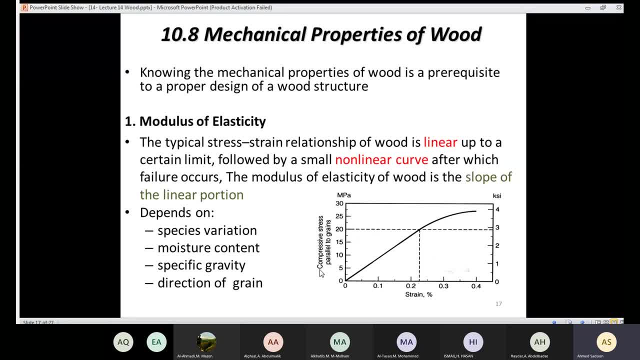 and then we are going to measure the force and the elongation, then we are going to determine which course of acceleration we are going to use here, because we are using a sphere cholera wicked in terms of plastics. so this one, as you was saying, like this one, has weights in the upper right. 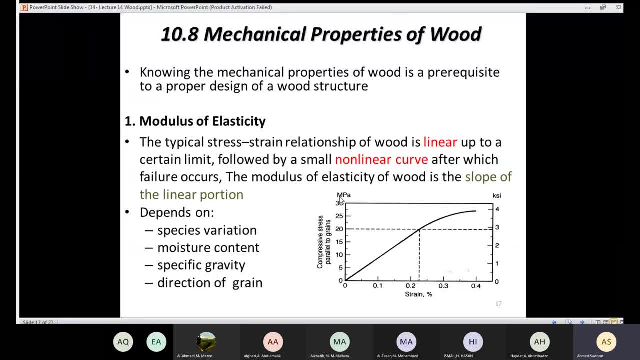 hand side in line with the weight of the weigh. the weight of the weighing inside of this thing actually vi assets in the lower Buy limits their danger. so the working pressure increase again is increased and so on. but the the importance of equipment left over is our learnt at least. in my last class we were talking about two times. OK, this one has been conducted parallel to the grain. longitude and axis. 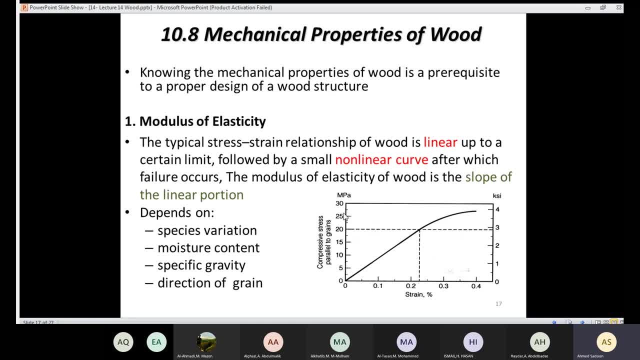 like that. the behavior is going to be similar, but the value of the modulus of elasticity is going to be different. so it's going to be linear up to a certain limit. after that we're going to have non-linear behavior. before the failure is how the stress strain diagram. look for the wood, okay, and 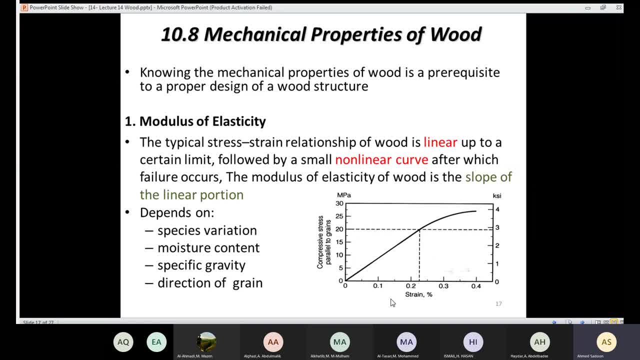 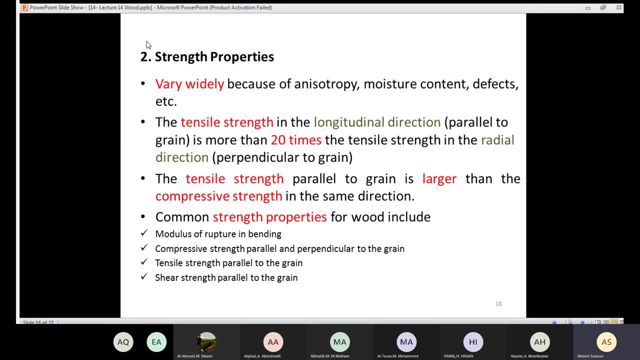 of course, the modulus of elasticity is the slope of the linear portion and that value depends on the species variation, it depends on the moisture content, it depends on the specific gravity and, of course, it depends on the direction of the grain. regarding the strings properties, again the strength property is going to vary. 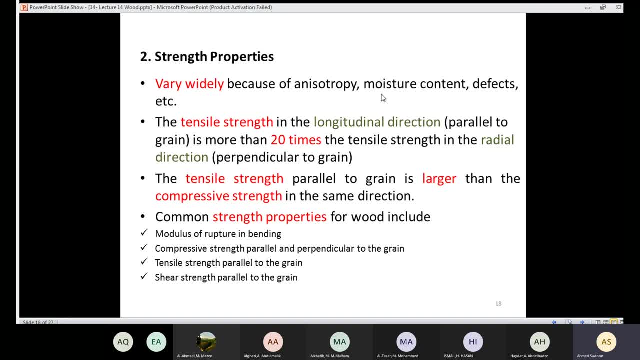 widely because of anisotropy and the moisture content and the defects. okay, the tensile strings in the longitudinal direction, the direction that parallel to the grain, is more than 20 times the tensile strength in the radial direction. so the the tensile strings is the 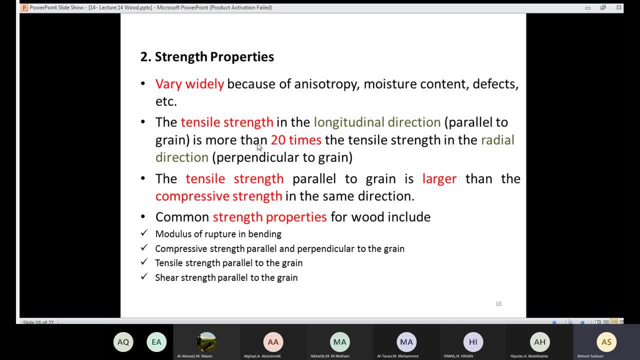 strongest in the longitudinal direction and it's about 20 times than the uh. the tensile strings in the radial direction, which is perpendicular to the grain- also, the tensile strings parallel to the grain- is larger than the compressive strings in the same direction. so if in the same direction these tensile strings is larger than the compressive string, 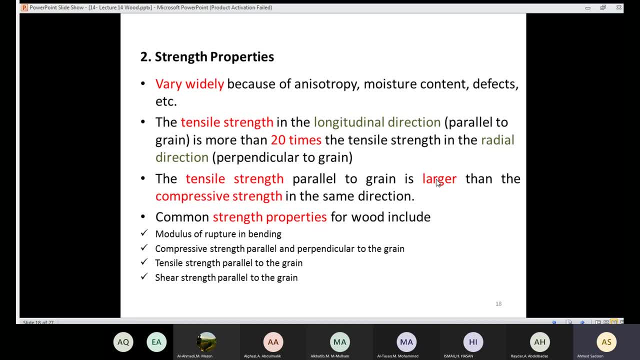 so in the wood the tensile strength is larger than the compressive string in the same direction. so here we have common strings properties for the wood. of course the modulus of rupture in bending, the compressive strings parallel and perpendicular to the grain, the tensile strings parallel to the grain and the shear strength parallel to the grain. 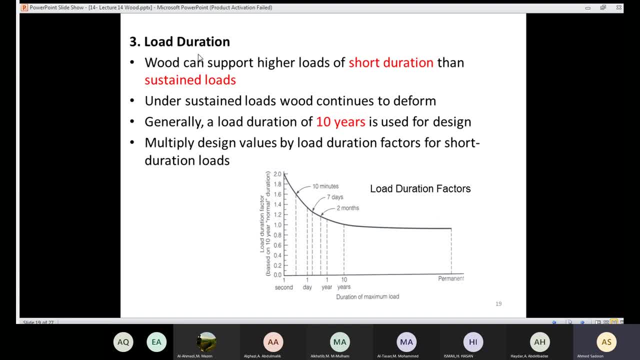 also, it's very important to talk about the load duration, because here we have strange phenomena regarding the, the wood, because wood can support a higher load of a short duration than a sustained load. for example, if you, if you have a piece of wood and then you apply a force to it, then the, the capacity after 10 minutes is going to be reduced. 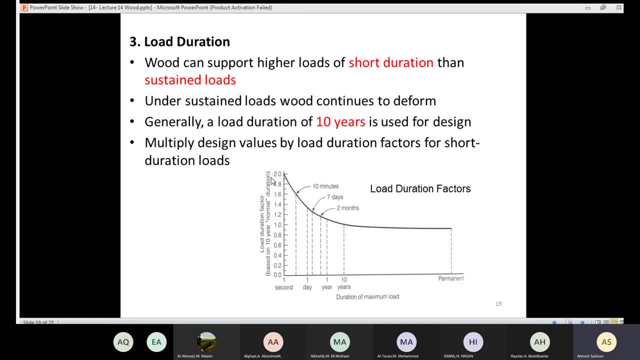 okay if the let's say that in the beginning the, the strings is two. okay, then, after 10 minutes, the strings is going to be 1.6. after seven days, the strength is going to be 1.3. after two months, the strength is going to be 1.2. after 10 years, the strength is going to be 1. 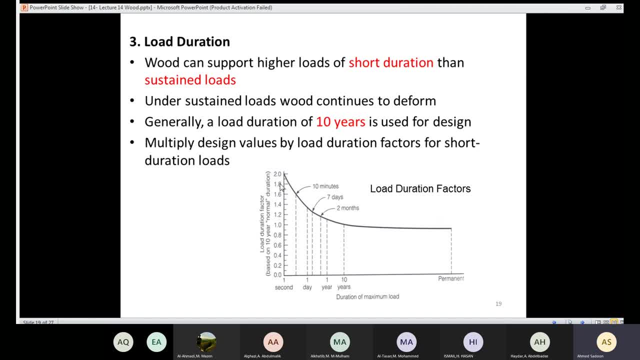 which means that after 10 years of sustained load, the the capacity of the wood is going to be reduced by half. okay, so this is the very strange phenomenon in the wood: it can support a higher load of a short time. for a short time it can. the capacity is high. 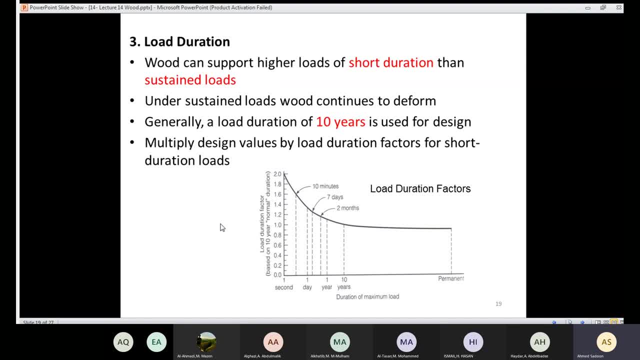 but after a long time, then the capacity is going to be reduced, like you can see here. that is why we generally we, uh, we design for a lot duration of 10 years in the design. so if you, if you are going to design a wood, you are going to design for a duration of 10 years. okay, if you wanna, if you are. 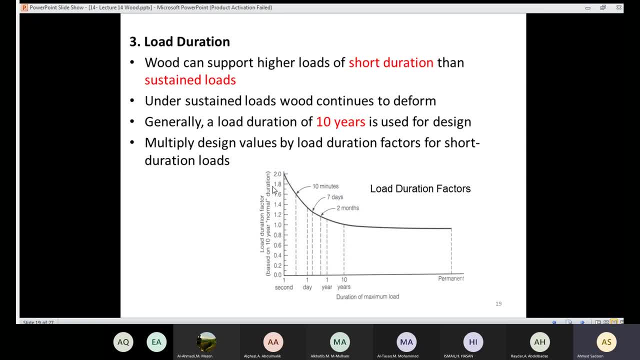 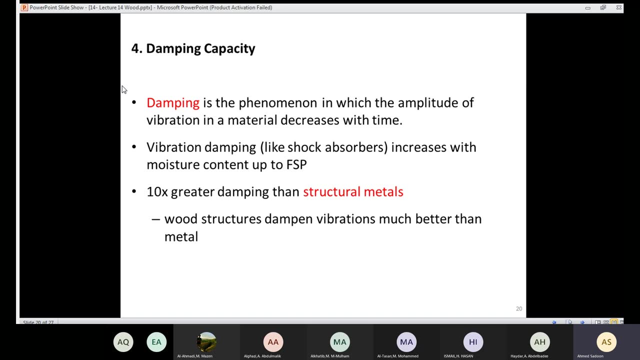 going to wait for 10 years to know the capacity. here you have the factors and you can use those factors in order to know the factor of safety. also, we have the dumping capacity. when we say dumping is the phenomenon in which the amplitude of the vibration in the material decreases with the time, okay, so the vibration dumping like shock. 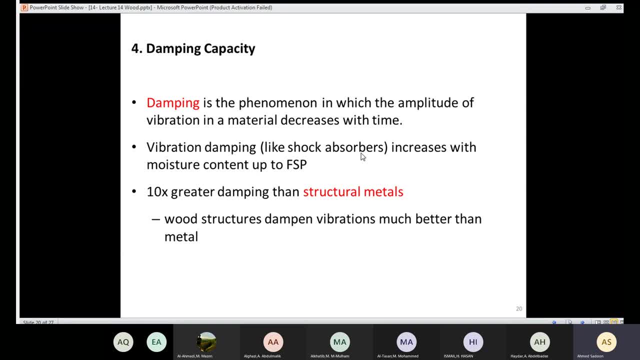 when we say that the material has good dumping, which means that it can absorb the, the shock, okay. for example, if you have, if the building is going to be hit by earthquake, then they are not. they are going to absorb that shock, okay. so the vibration dumping for the wood increases with the 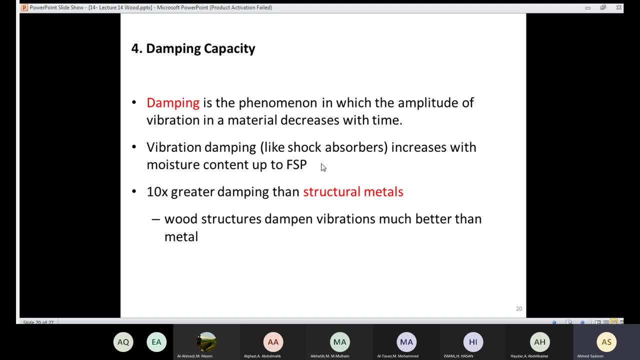 moisture content up to fsb. so when the moisture content increase, the dubbing process is going to increase as well. and surprisingly, the dumping capacity for the wood is 10 times greater- greater than the structural metal, which means that the wood structure dumping vibration much better than 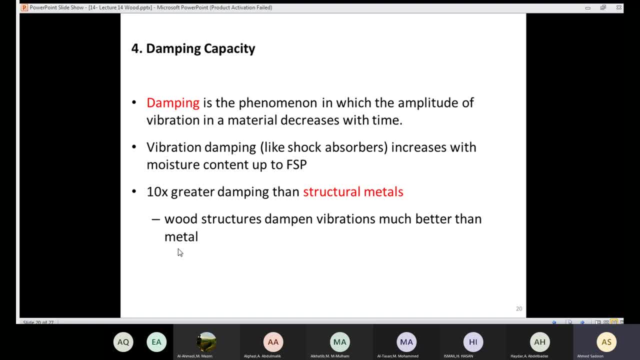 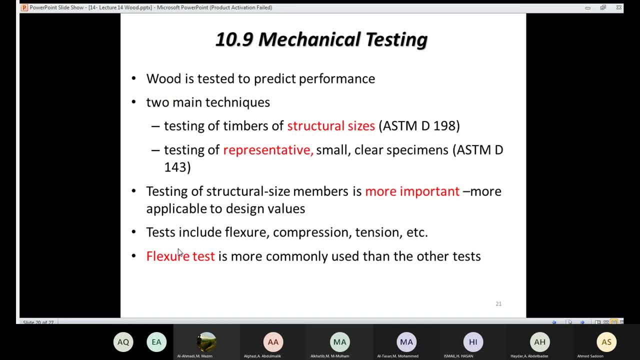 the metal, so the wood. it has good resistance for damping than the, than the steel and aluminium and so on. now we need to talk about the mechanical testing itself. we will talk about energy processing itself, how to test, which type of test should be conducted in order to know the mechanical? 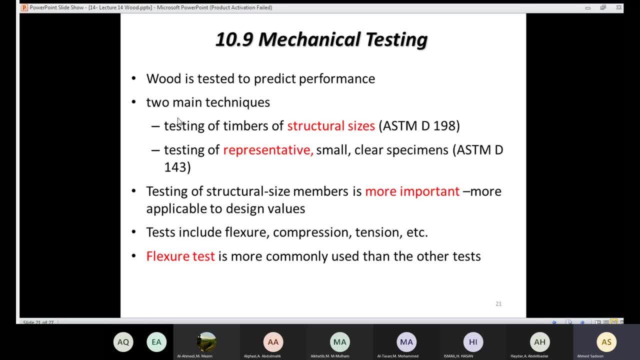 properties of the wood. we have two main techniques. okay, testing of a timber of structural sizes. okay, which means that we are gonna test the, the, the, the, the, the same size that is going to be used on the side. or you can take representative sample, which means that you are going to take only small. 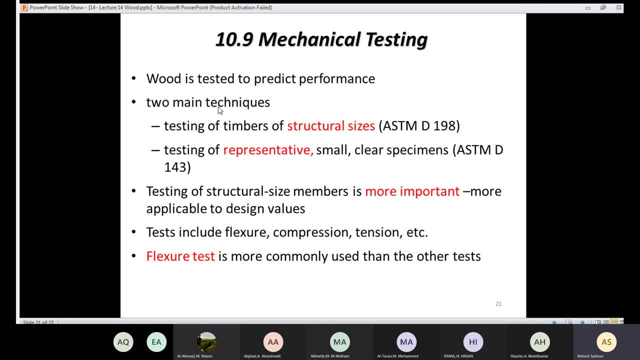 sample okay. so which one is important? of course, testing the actual size is very important than the representative okay, because this one is going to be close to reality. so testing of structural size, members, is more important, more applicable to the design values. we have tests like structural: we have the flexure test, we have the compression test, we have the tension test, the most important. 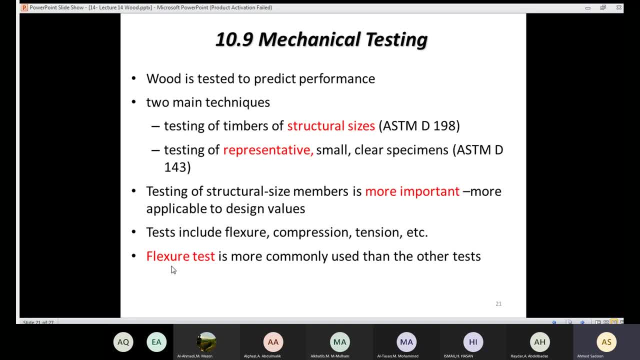 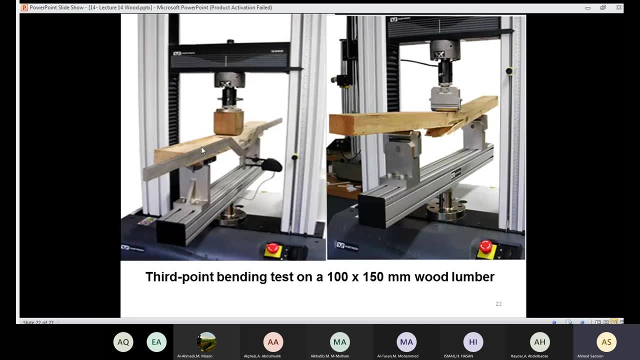 test is a flexure test is more commonly used than the other test, mainly because of the. the tensile strength of the wood is the, the most dominant value. here we have example for flexural test. here we we have an actual size of the wood and here we put a force in the middle so that we can determine the value of the flexural strength. 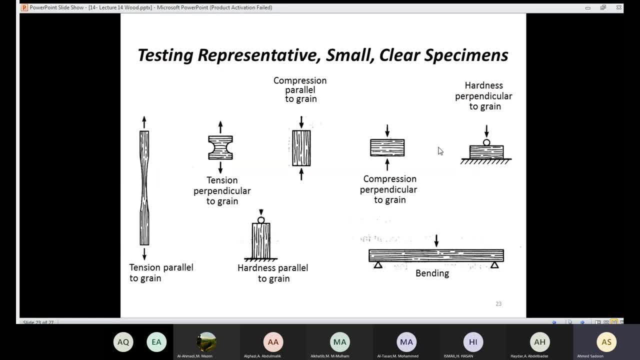 okay, so is it this look like? here we have a representative sample, if you want to take a small sample. so here we have a representative sample. of course, remember we, for example, for example, if you want to contact compressive strength, this one is, for example, should be parallel to the grain and you need to another one which is perpendicular to 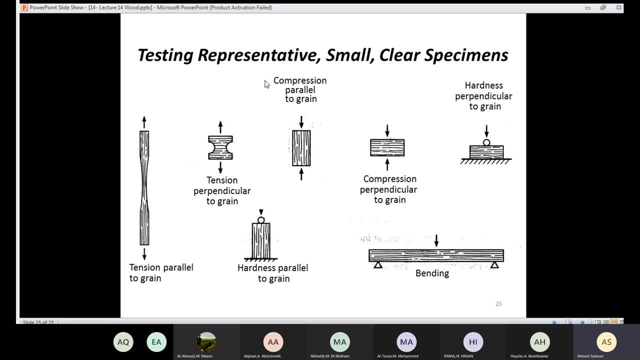 the grain, because we say that the wood is anaestropic. the properties is going to be different from one direction to another. so each and every test should be first conducted parallel to the grain and also should be conducted perpendicular to the grain. here, for example, for tension test should be perpendicular to the grain and also should be parallel to the grain. 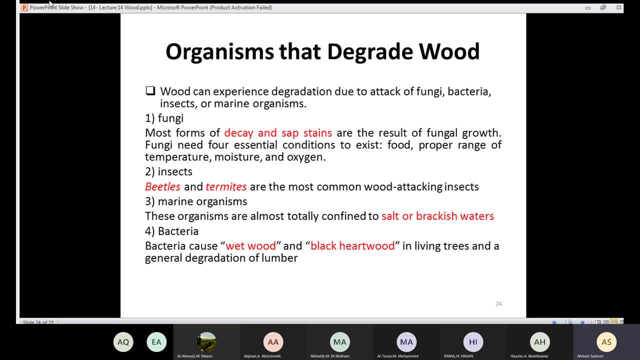 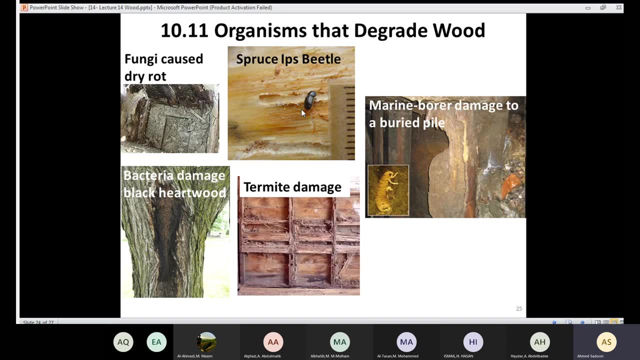 so, finally, we need to talk about the organisms that that degrade the wood. the wood can experience degradation due to attack of fungi, bacteria, insect or marine organisms like that. the the wood is susceptible to fungi and insects and insects from the marine, and that could degrade the wood okay. 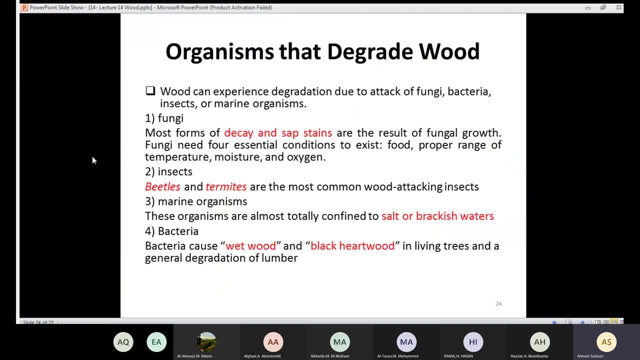 first, we have the fungi. the most form of decay and sap stain a result of fungal growth. so the most damage that you could seen is going to be as a result of a fungi. okay, so fungi, in order to exist, you need to have a food, you need to have a proper range of temperature, you need to have a moisture and we need to have oxygen. 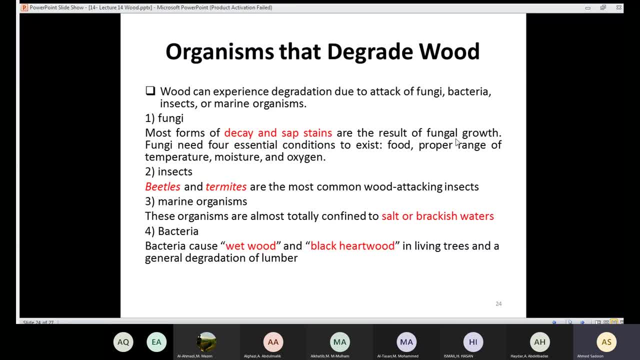 so if you want to get rid of the fungi, you need to make sure that one of these is not existed. also, we have insects: we have the beetles and we have the termites- this one are the most common wood attacking insects- and also we have, uh uh, marine organisms. this organism almost almost totally confined to salt or brackish. 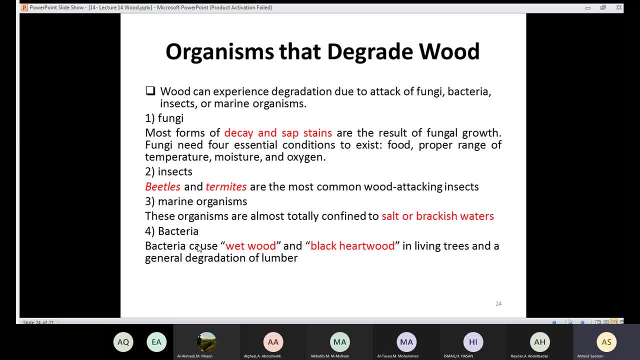 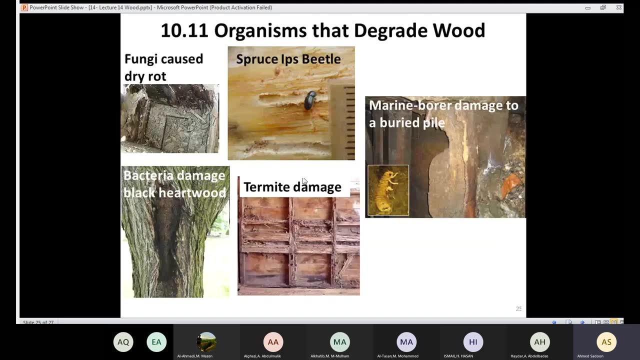 waters and finally we have the bacteria. the bacteria cause the wet wood and a black, a hard wood in living trees and a general degradation of alumber bacteria that's going to cause the black heart wood. here we have the termite damage, here we have the beetle damage, here we have damage due to fungi and here we have a damage due to marine insects. 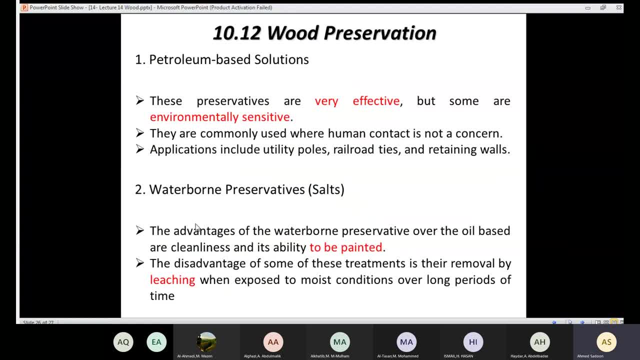 finally, in order to prevent the wood from all of this, we have two type of solutions. we have petroleum-based solution and we have waterborne preservative, which is made from salts. okay, the petroleum-based solution- this one is- is very effective, but this one is environmentally sensitive. it's going to hurt the environment. usually, we use this petroleum-based solution.